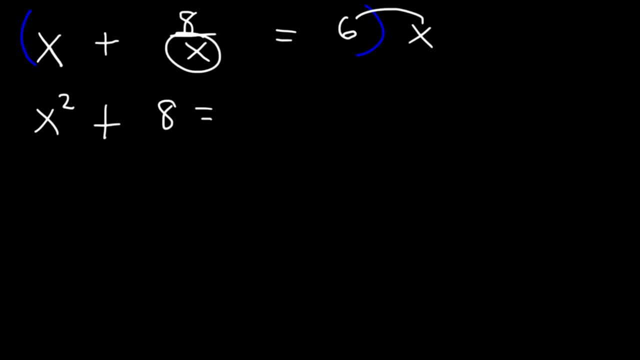 Next, x times 6 is basically 6x. So now what you want to do at this point. you want to subtract both sides by 6x. Well, basically, just take this term and move it to the left side. Since we now have a quadratic equation, It's positive 6x on the right side, but on the left side it's going to be negative 6x. And let's put it in standard form. 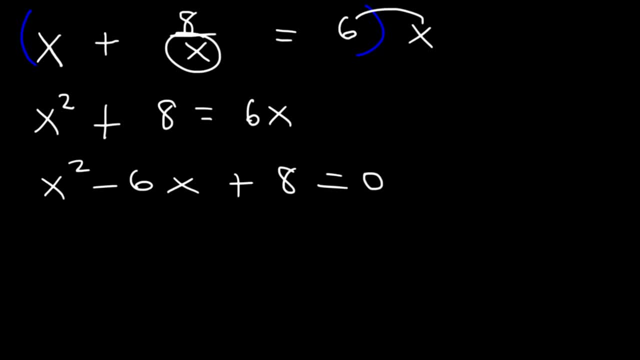 So now, what would you do in order to solve this equation? Solve for x. at this point, Whenever you have a quadratic function like this, you can either factor it or use the quadratic equation to solve for x. Let's factor the expression: What two numbers multiply to 8, but add to the middle coefficient negative 6?? 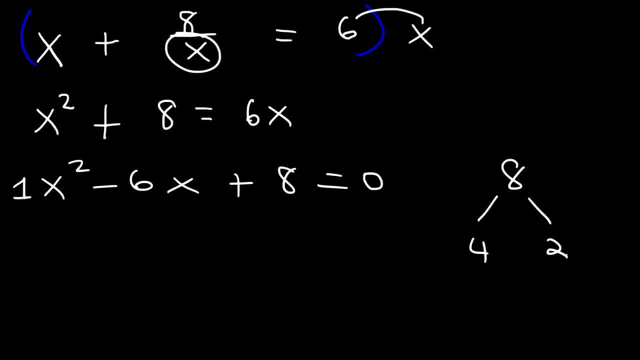 Well, we know that 4 times 2 is equal to 8,, but 4 plus 2 is positive 6.. However, if we add the middle coefficient to the middle coefficient, we get negative 6.. If we add two negative signs, negative 4 times negative, 2 is still positive 8, but it adds to negative 6.. 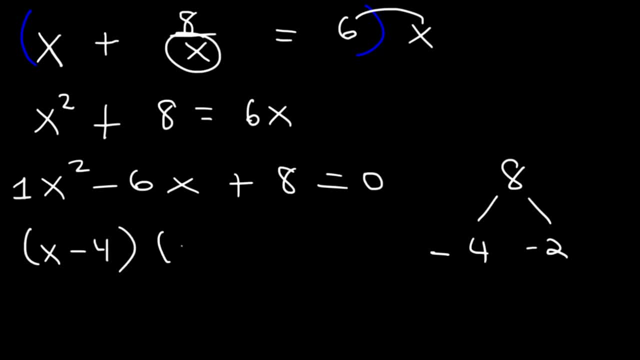 So to factor it, it's going to be x minus 4 times x minus 2.. Now what you need to do next is to set each factor equal to 0 and solve for x. So in the first equation, if we add 4 to both sides, we can see that x is equal to 4.. 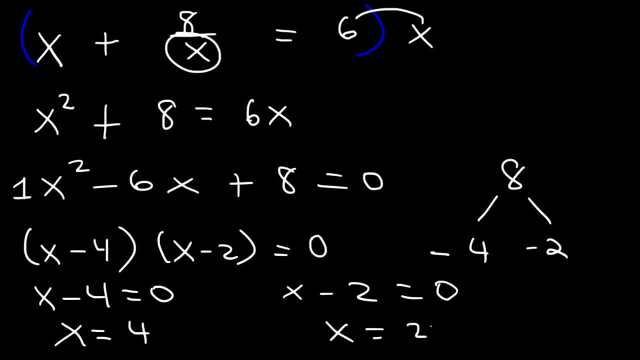 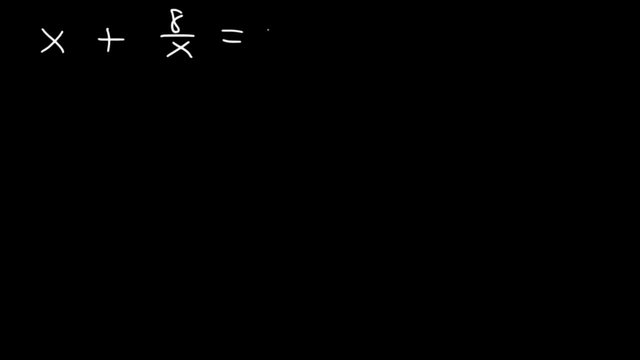 And in the second one, if we add 2 to both sides, we can see that x is equal to 2.. So now let's check these answers to make sure that they both work, Because sometimes you may have extraneous solutions. So the original equation is: x plus 8 over x is equal to 6.. 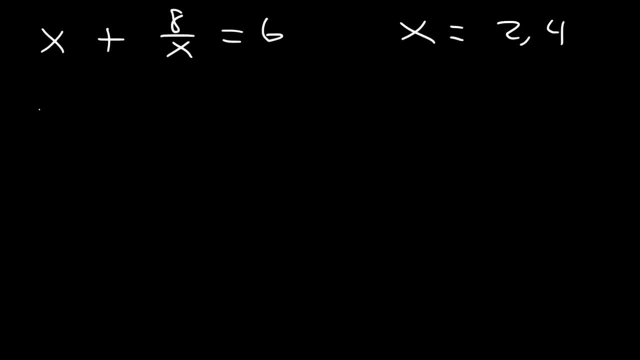 And we have two answers: 2 and 4.. Let's try 2.. So 2 plus 8 divided by 2, is that equal to 6?? 8 divided by 2 is 4.. 2 plus 4 is 6.. 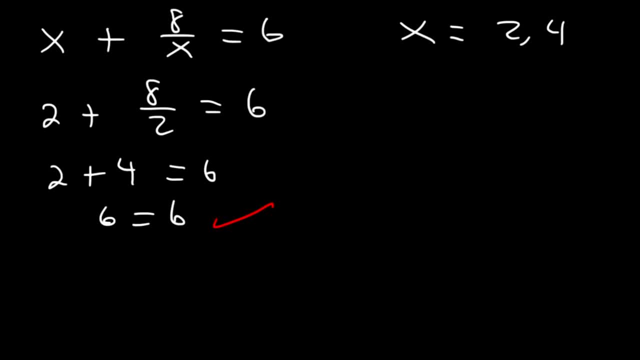 So that works. Now what if we plug in 4? 4 plus 8 over 4, does that equal to 6? 8 divided by 4 is 2.. 4 plus 2 is 6.. And so this works as well. 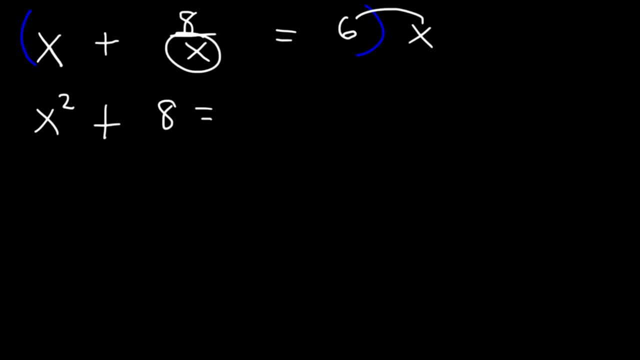 Next, x times 6 is basically 6x. So now what you want to do at this point. you want to subtract both sides by 6x. Well, basically, just take this term and move it to the left side. Since we now have a quadratic equation, It's positive 6x on the right side, but on the left side it's going to be negative 6x. And let's put it in standard form. 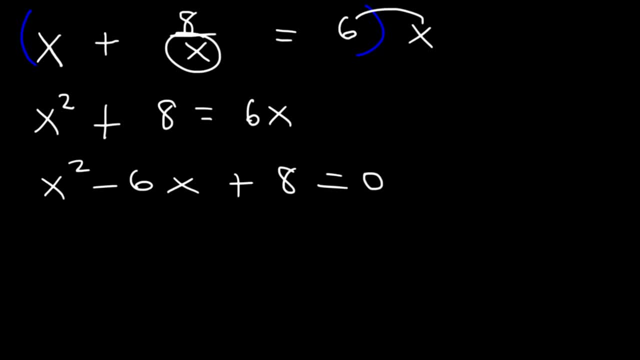 So now, what would you do in order to solve this equation? Solve for x. at this point, Whenever you have a quadratic function like this, you can either factor it or use the quadratic equation to solve for x. Let's factor the expression: What two numbers multiply to 8, but add to the middle coefficient negative 6?? 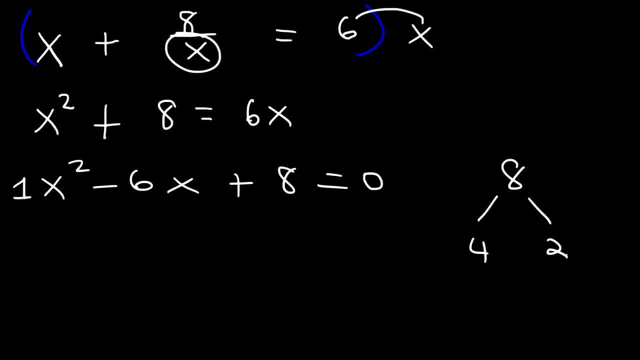 Well, we know that 4 times 2 is equal to 8,, but 4 plus 2 is positive 6.. However, if we add the middle coefficient to the middle coefficient, we get negative 6.. If we add two negative signs, negative 4 times negative, 2 is still positive 8, but it adds to negative 6.. 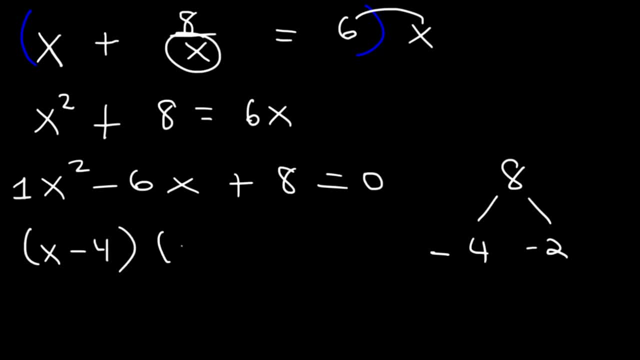 So to factor it, it's going to be x minus 4 times x minus 2.. Now what you need to do next is to set each factor equal to 0 and solve for x. So in the first equation, if we add 4 to both sides, we can see that x is equal to 4.. 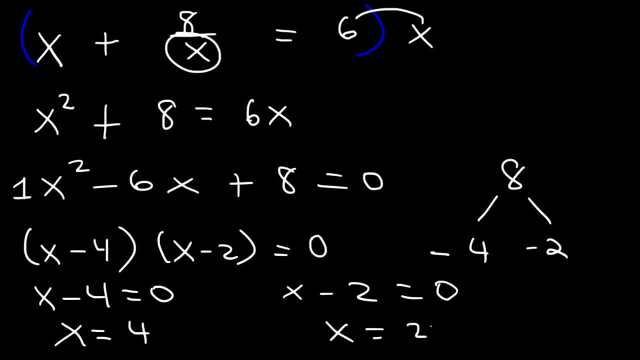 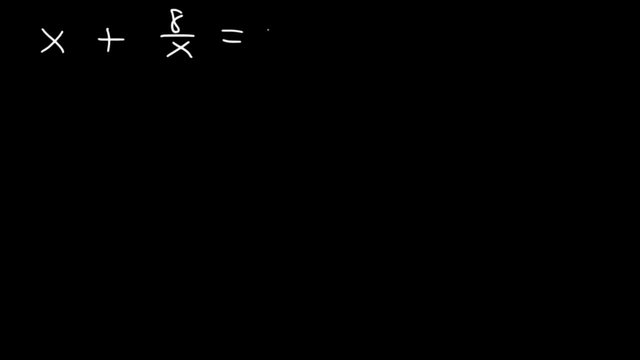 And in the second one, if we add 2 to both sides, we can see that x is equal to 2.. So now let's check these answers to make sure that they both work, Because sometimes you may have extraneous solutions. So the original equation is: x plus 8 over x is equal to 6.. 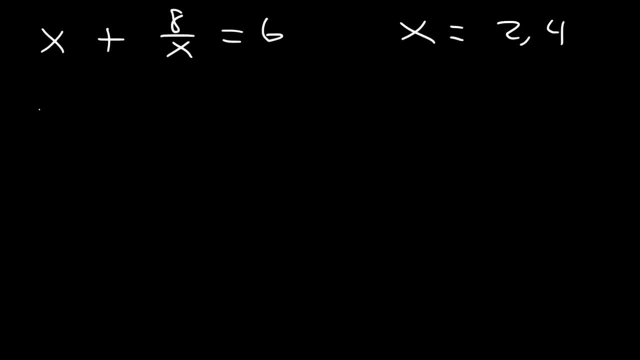 And we have two answers: 2 and 4.. Let's try 2.. So 2 plus 8 divided by 2, is that equal to 6?? 8 divided by 2 is 4.. 2 plus 4 is 6.. 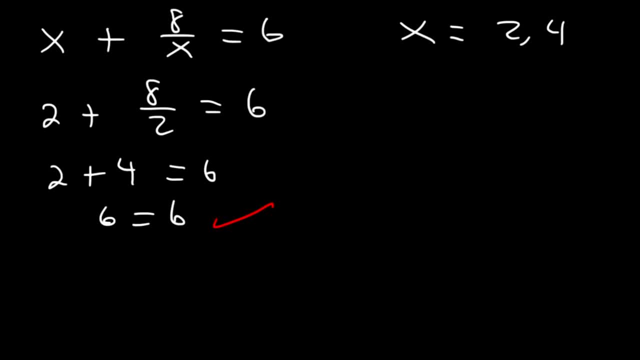 So that works. Now what if we plug in 4? 4 plus 8 over 4, does that equal to 6? 8 divided by 4 is 2.. 4 plus 2 is 6.. And so this works as well. 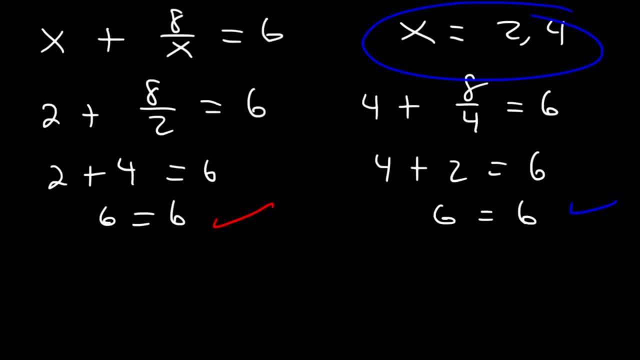 So x is indeed equal to 2 or 4.. Now let's work on another example. Let's try this one. Let's say that 3x plus 4, divided by x minus 1, is equal to 11. Go ahead and solve for the variable x. 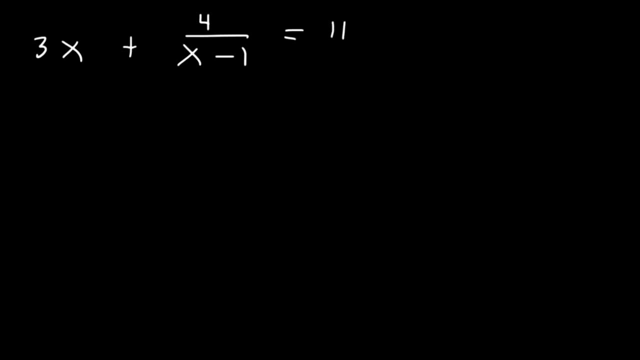 So what do you think we have to do in this particular problem? Well, like the other problem, we need to clear away the fractions. So let's multiply both sides by x, x minus 1.. So we're going to have 3x times x minus 1.. 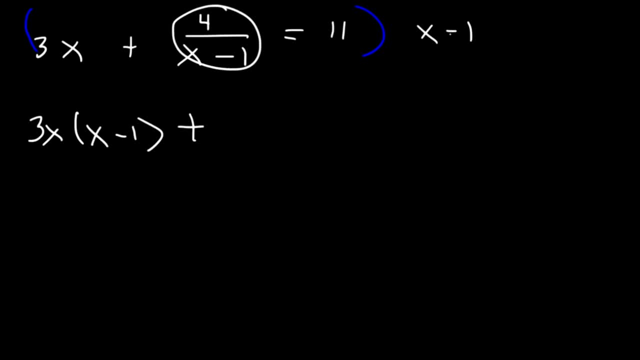 And then, if we multiply 4 over x minus 1 by x minus 1, these two will cancel and we're just going to get 4.. And then we have 11 times x minus 1.. So now that we no longer have any fractions to deal with. 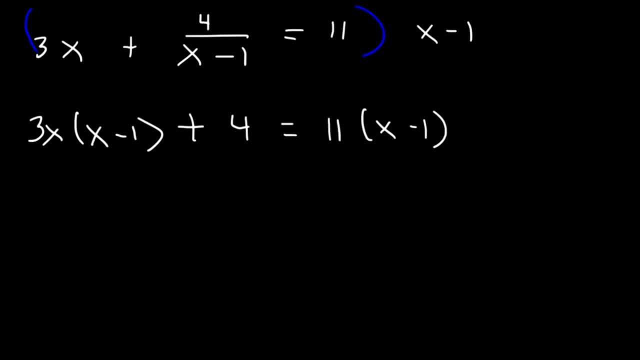 let's distribute and then combine like terms. So 3x times x, that's going to be 3x squared. And then if we multiply 3x by negative 1, that's negative 3x, and then plus 4.. 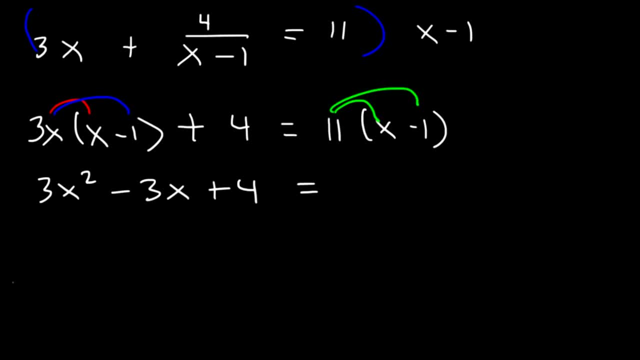 Now let's distribute 11 to x and to negative 1. So on the right side that's going to be 11x minus 11.. So now, everything that's on the right side. let's move it to the left side. 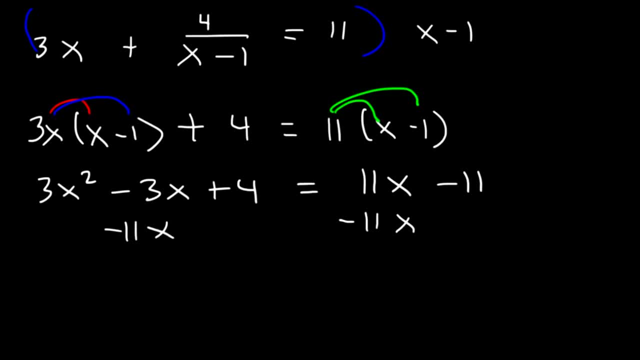 So let's subtract both sides by 11x And at the same time let's add 11 to both sides, So we're going to have nothing left over on the right side, And then on the left side it's going to be 3x squared. 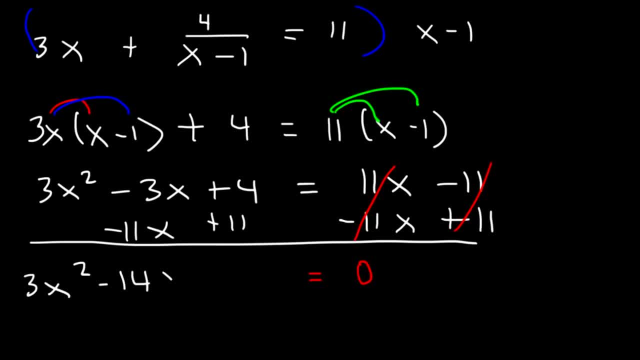 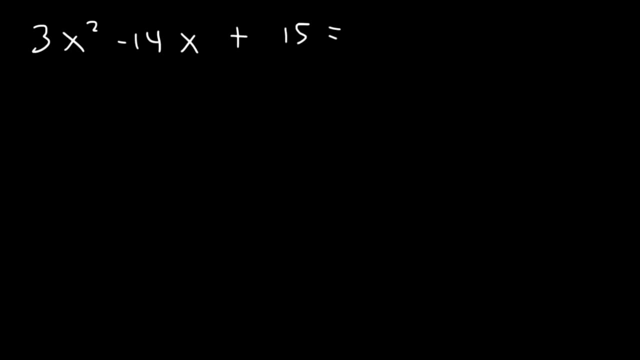 negative. 3x minus 11x, that's negative 14x, And 4 plus 11 is 15.. So we have 3x squared minus 14x. plus 15 is equal to 0.. Now let's solve for x. 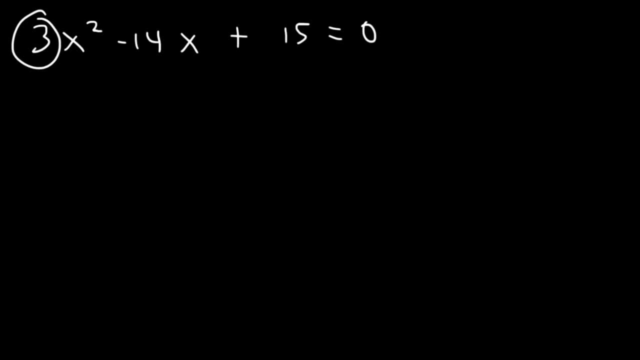 So here we have a trinomial where the leading coefficient is 1.. So to factor it it's going to require a little bit more work. The first thing we need to do is multiply the leading coefficient by the constant term. 3 times 15 is 45.. 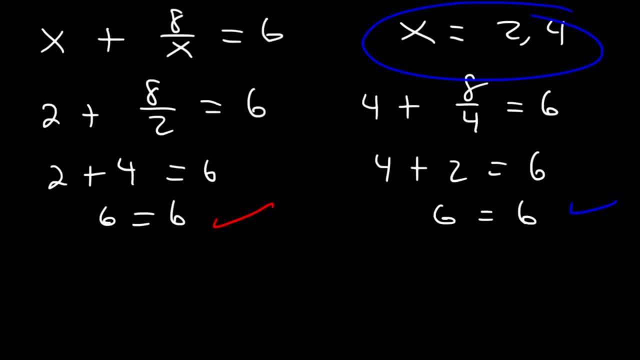 So x is indeed equal to 2 or 4.. Now let's work on another example. Let's try this one. Let's say that 3x plus 4, divided by x minus 1, is equal to 11. Go ahead and solve for the variable x. 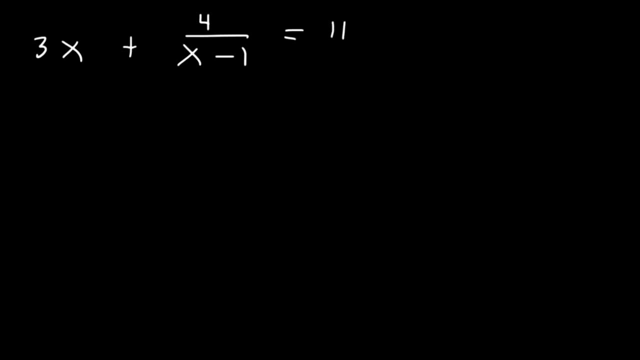 So what do you think we have to do in this particular problem? Well, like the other problem, we need to clear away the fractions. So let's multiply both sides by x, x minus 1.. So we're going to have 3x times x minus 1.. 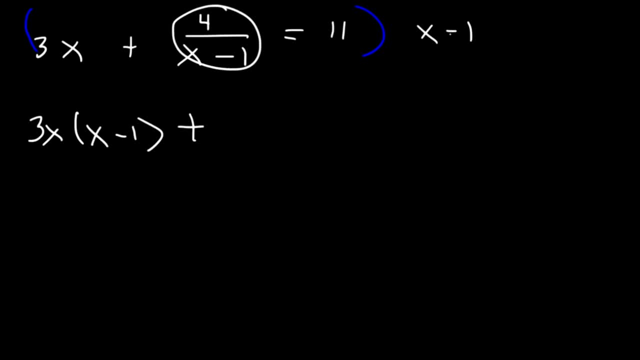 And then, if we multiply 4 over x minus 1 by x minus 1, these two will cancel and we're just going to get 4.. And then we have 11 times x minus 1.. So now that we no longer have any fractions to deal with. 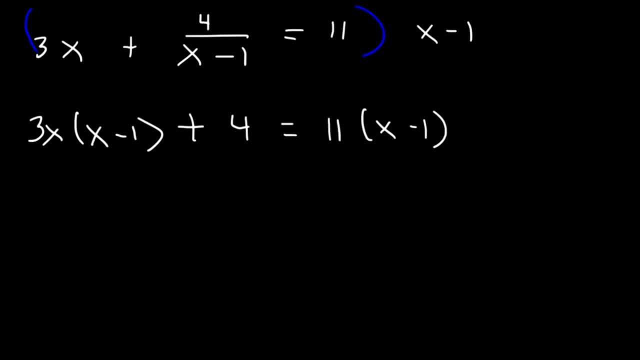 let's distribute and then combine like terms. So 3x times x, that's going to be 3x squared. And then if we multiply 3x by negative 1, that's negative 3x, and then plus 4.. 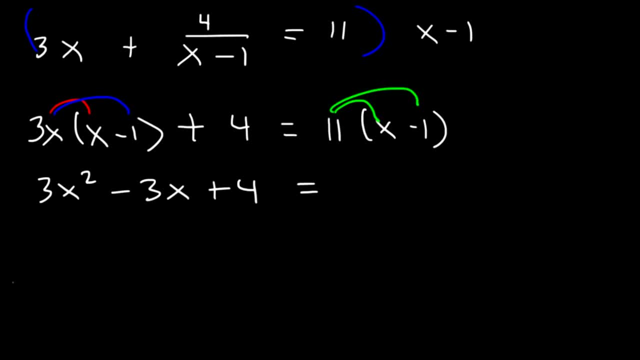 Now let's distribute 11 to x and to negative 1. So on the right side that's going to be 11x minus 11.. So now, everything that's on the right side. let's move it to the left side. 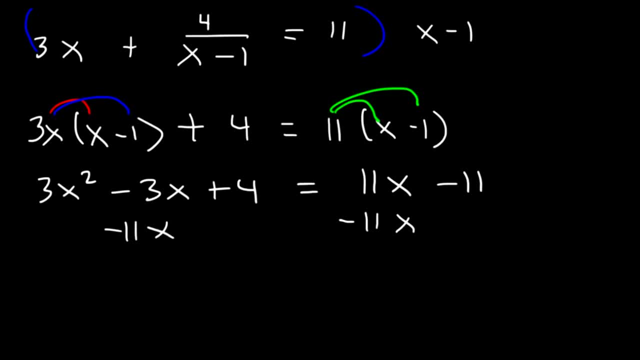 So let's subtract both sides by 11x And at the same time let's add 11 to both sides, So we're going to have nothing left over on the right side, And then on the left side it's going to be 3x squared. 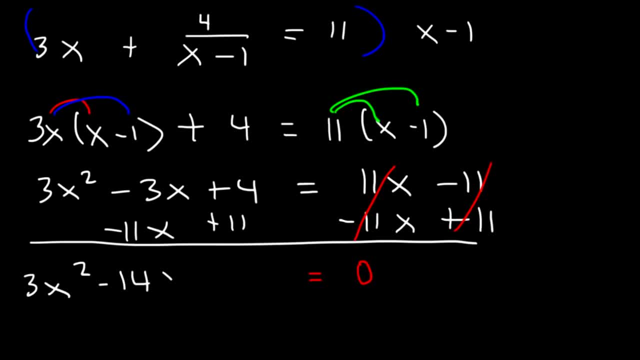 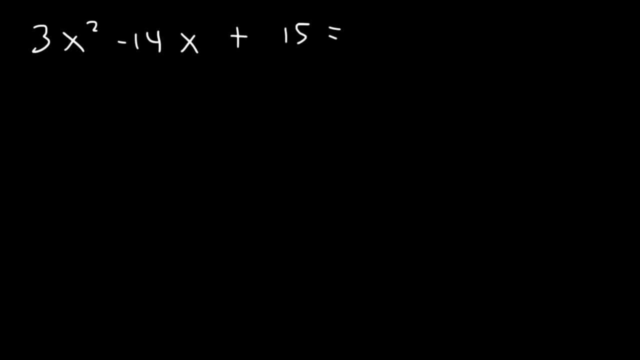 negative. 3x minus 11x, that's negative 14x, And 4 plus 11 is 15.. So we have 3x squared minus 14x plus 15, that's 0.. Now let's solve for x. 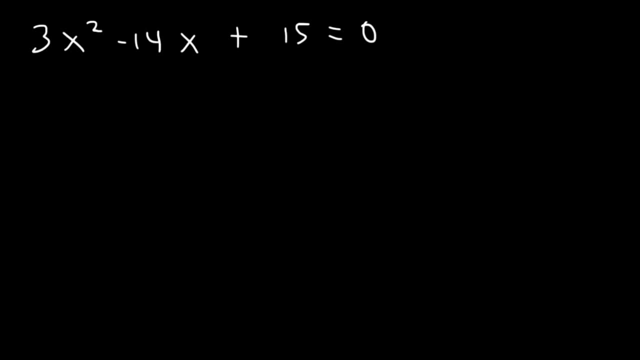 So here we have a trinomial where the leading coefficient is 1.. So to factor it it's going to require a little bit more work. The first thing we need to do is multiply the leading coefficient by the constant term. 3 times 15 is 45.. 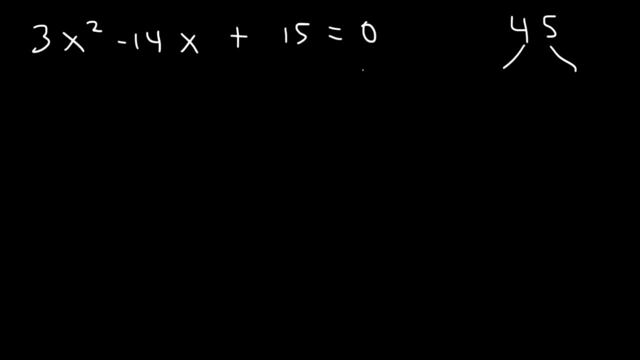 3 times 15 is 45.. to find two numbers that multiply to 45, but add to negative 14.. Well, we know that 5 times 9 is 45.. 5 plus 9 is 14.. We just got to make it negative. Now what you need to do at this point. 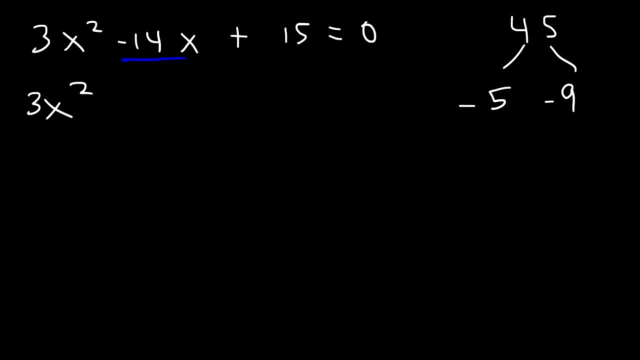 is: replace the middle term negative 14x with negative 9x and negative 5x. The order in which you write it really doesn't matter, but I prefer to put 3 and 9 because it's easy to see what the 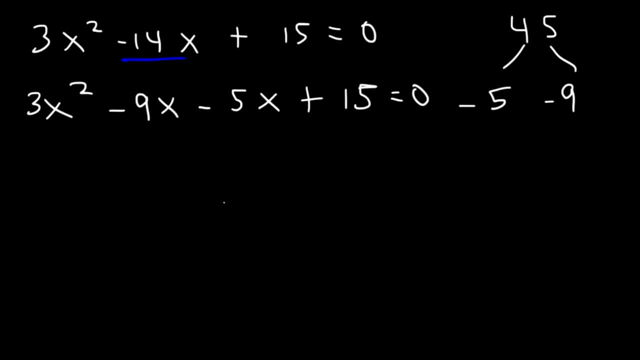 multiple is or the GCF: 3 can go to 3 and 9, and 5 can go into 5 and 15.. Now what we need to do at this point is we need to factor by grouping. We need to take out the GCF in the first two terms. 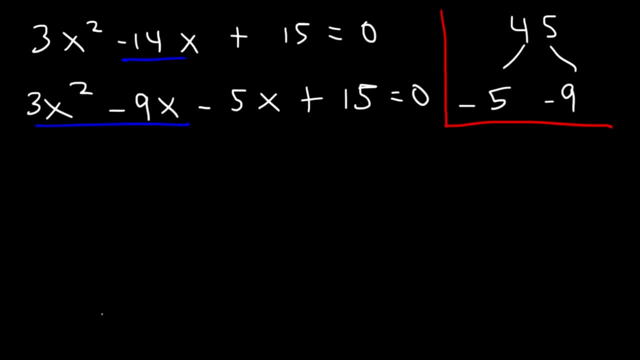 The greatest common factor between 3x squared and negative 9x is 3x. To find out what goes inside the parentheses, simply divide 3x squared. divided by 3x is x and negative 9x divided by 3x is negative 3.. Now for the last two terms. 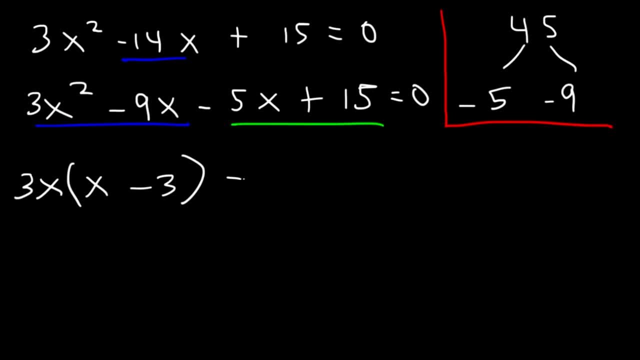 you can do the same thing. Take out the GCF. In this case, it's going to be negative 5.. Negative 5x divided by negative 5 is positive x. 15 divided by negative 5 is negative 3.. 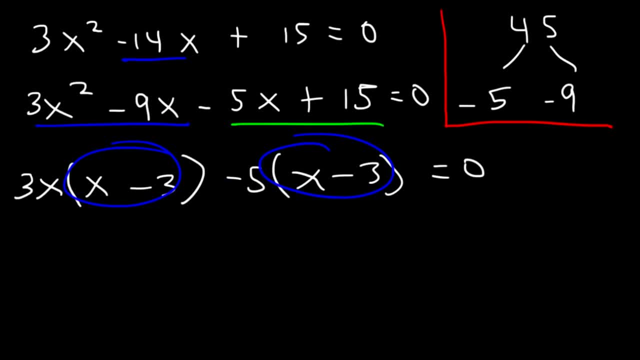 Now, if these two factors are the same, then you've done it correctly up to this point. So now we're going to factor out the GCF from these two terms, which is x minus 3.. So when you factor it out, you only need to write it once. 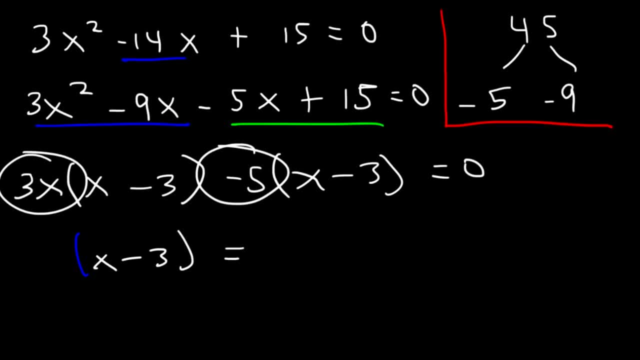 And on the outside we have a 3x and a negative 5.. So x minus 3 times 3x minus 5 is equal to 3x squared minus 4x plus 15.. So now let's set each factor equal to 0.. 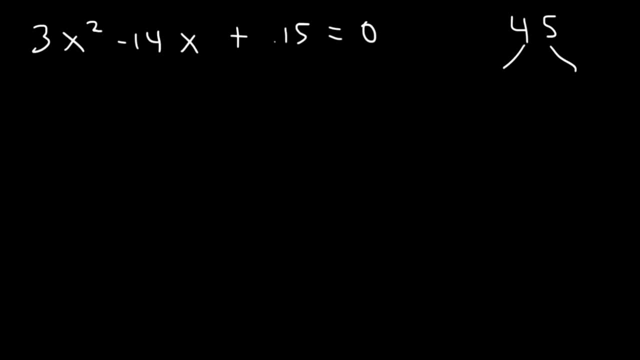 Now we need to multiply the leading coefficient by the constant term to find two numbers that multiply to 45, but add to negative 14.. Well, we know that 5 times 9 is 45.. 5 plus 9 is 14.. We just got to make a negative. Now what you need to do at this point? 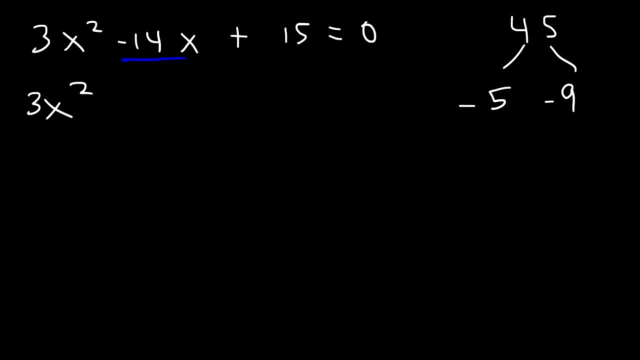 is: replace the middle term negative 14x with negative 9x and negative 5x. The order in which you write it really doesn't matter, but I prefer to put 3 and 9 because it's easy to see what the 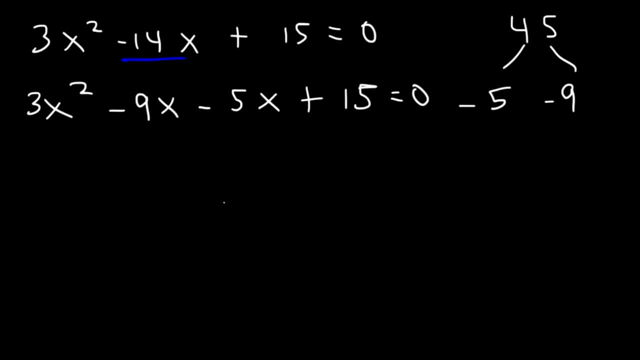 multiple is or the GCF: 3 can go to 3 and 9, and 5 can go into 5 and 15.. Now what we need to do at this point is we need to factor by grouping. We need to take out the GCF in the first two terms. 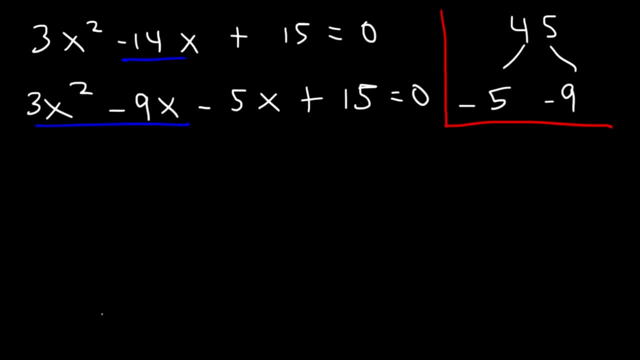 The greatest common factor between 3x squared and negative 9x is 3x. To find out what goes inside the parentheses, simply divide 3x squared. divided by 3x is x and negative 9x divided by 3x is negative 3.. Now for the last two terms. 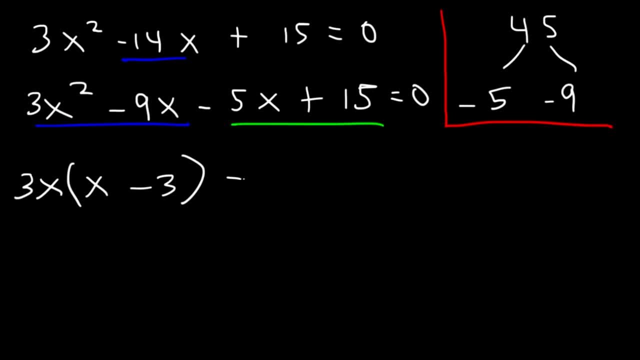 you can do the same thing. Take out the GCF. In this case, it's going to be negative 5.. Negative 5x divided by negative 5 is positive x. 15 divided by negative 5 is negative 3.. 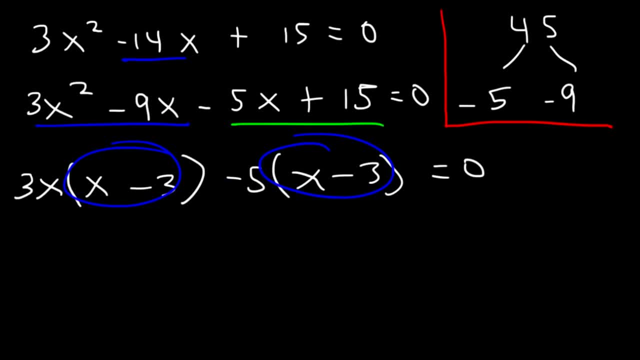 Now, if these two factors are the same, then you've done it correctly up to this point. Now we're going to factor out the GCF from these two terms, which is x minus 3.. When you factor it out, you only need to write it once. 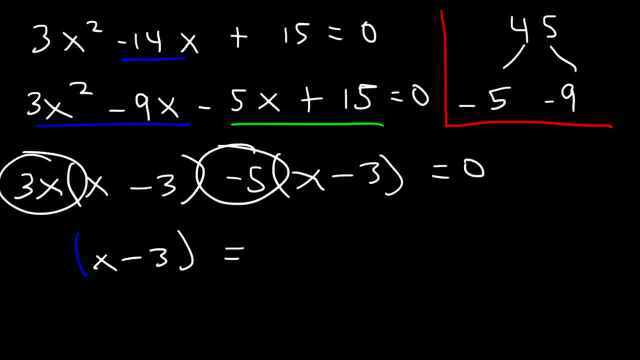 On the outside we have a 3x and a negative 5.. So x minus 3 times 3x minus 5 is equal to 3x squared minus 4x plus 15.. So now let's set each factor equal to 0.. 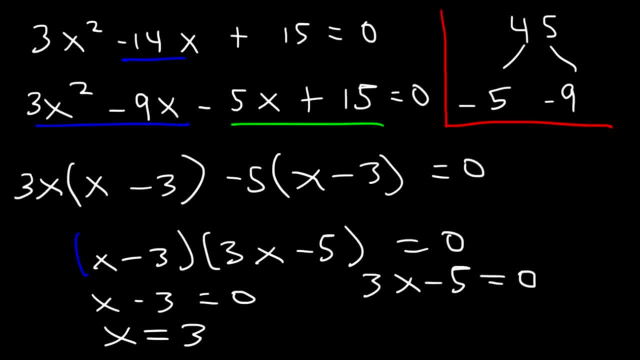 So on the left we can see that x is equal to 3.. That's the first answer, And on the right we need to add 5.. So 3x is equal to 5. And then divide both sides by 3.. So x is 5 over 3.. 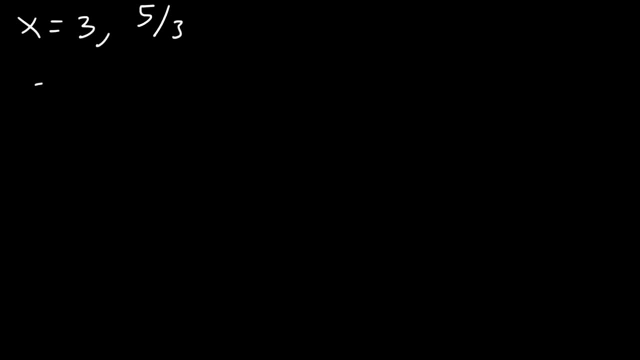 Now let's just check to make sure that both answers indeed work. So let's start with the first one. Let's replace x with 3.. So it's going to be 3 times 3 plus 4 over. 3 minus 1 is equal to 11.. 3 times 3 is 9.. And 3 minus 1 is 2.. 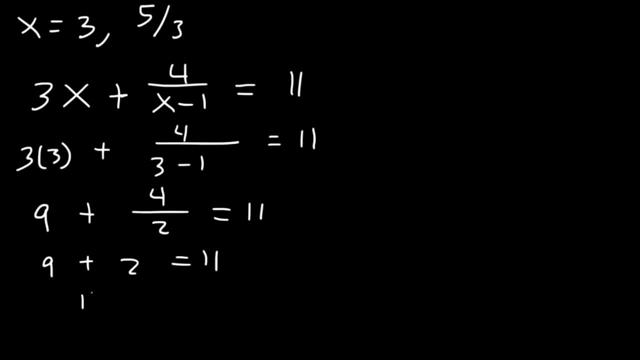 4 divided by 2 is 2.. 9 plus 2 is 11.. So 3 is indeed a solution. Now let's try 5 over 3. So we're going to have 3 times 5 over 3 plus 4.. 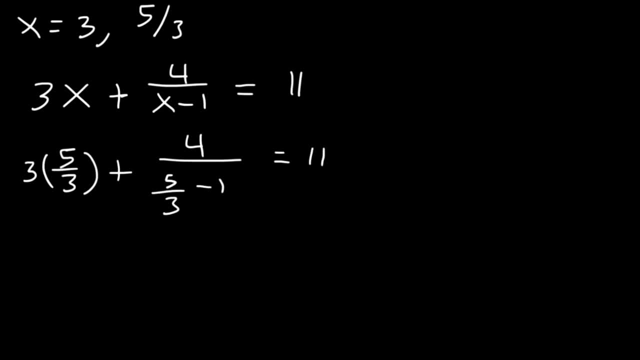 Divided by 5 over 3 minus 1 is equal to 11.. Well, 3 times 5, thirds, the 3s cancel and you're just going to get 5.. Next, we need to simplify this complex fraction. 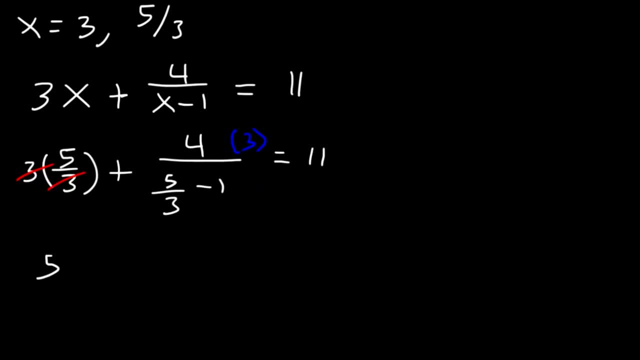 And the best way we can do that is to multiply the top and the bottom by 3.. On top, 4 times 3 is 12.. On the bottom, we need to distribute the 3. So 3 times 5 thirds: the 3s will cancel. 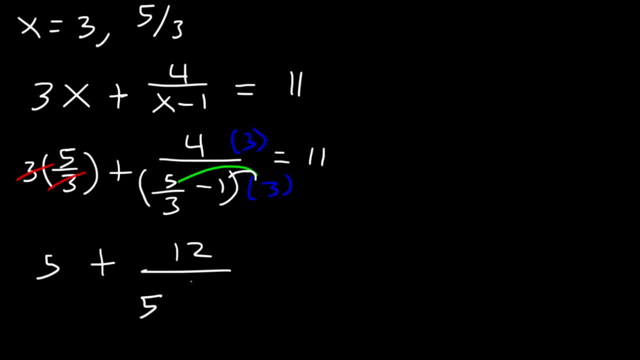 And you're just going to get 5. And then 3 times negative, 1 is negative 3. Now, 5 minus 3 is 2.. 12 divided by 2 is 6.. 5 plus 6 is 11.. 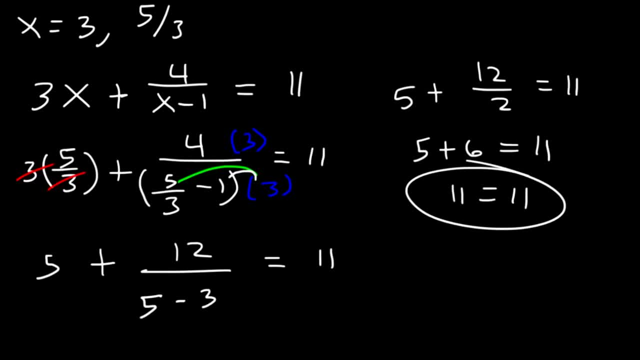 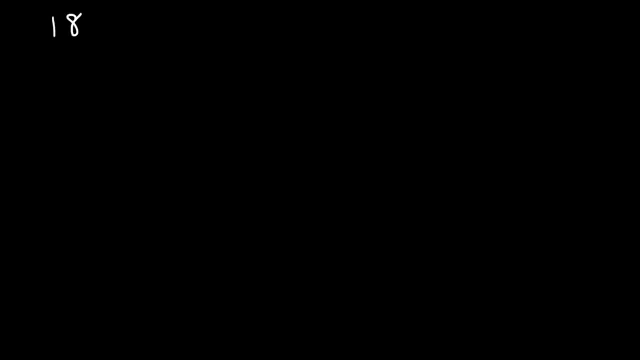 And so this works as well. Therefore, both answers are acceptable. Now, what if there are two fractions as opposed to one, Like this example? What should we do in this case? We have two different denominators. In a situation like this, what you want to do is you want to multiply both sides by the common denominator. 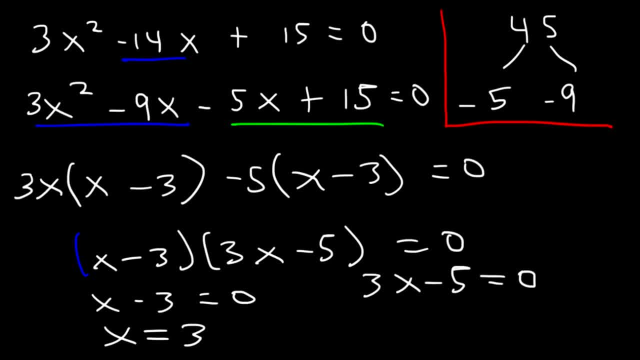 So on the left we can see that x is equal to 3.. That's the first answer, And on the right we need to add 5.. So 3x is equal to 5. And then divide both sides by 3.. So x is 5 over 3.. 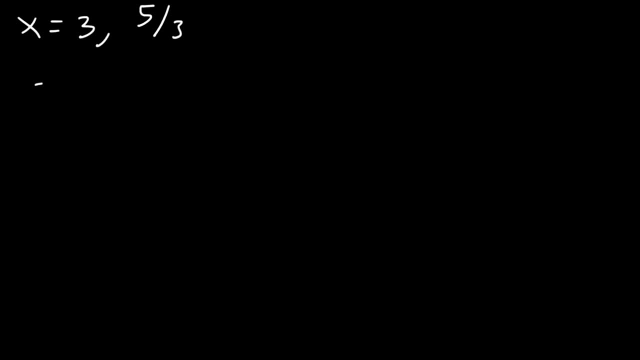 Now let's just check to make sure that both answers indeed work. So let's start with the first one. Let's replace x with 3.. So it's going to be: 3 times 3 plus 4 over. 3 minus 1 is equal to 11.. 3 times 3 is 9.. And 3 minus 1 is 2.. 4 divided by 2 is 2.. 9 plus 2 is 11.. 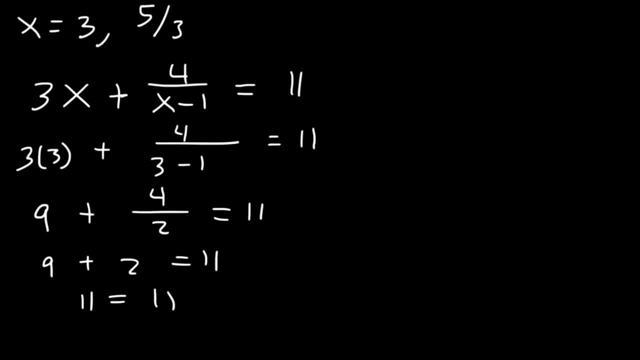 So 3 is indeed a solution. Now let's try 5 over 3.. So we're going to have 3 times 5 over 3 plus 4.. So we're going to have 3 times 5 over. 3 minus 1 is equal to 11.. 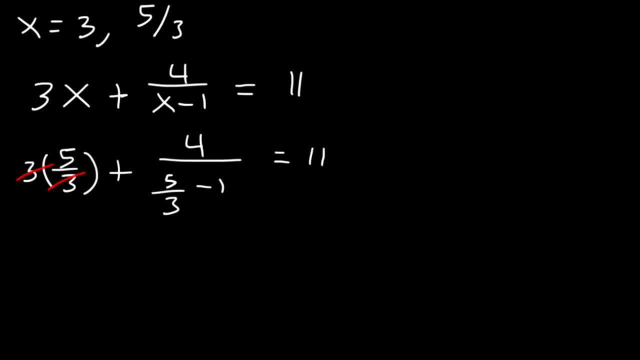 Well, 3 times 5, thirds, the 3's cancel and you're just going to get 5.. Next, we need to simplify this complex fraction, And the best way we can do that is to multiply the top and the bottom by 3.. 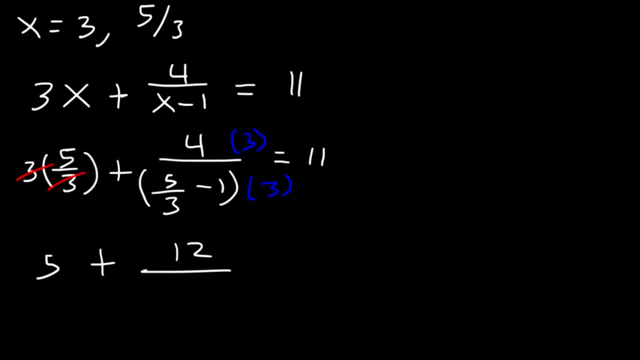 On top: 4 times 3 is 12.. On the bottom, we need to distribute the 3.. So 3 times 5, thirds, the 3's will cancel And you're just going to get 5.. And then 3 times negative: 1 is negative 3.. 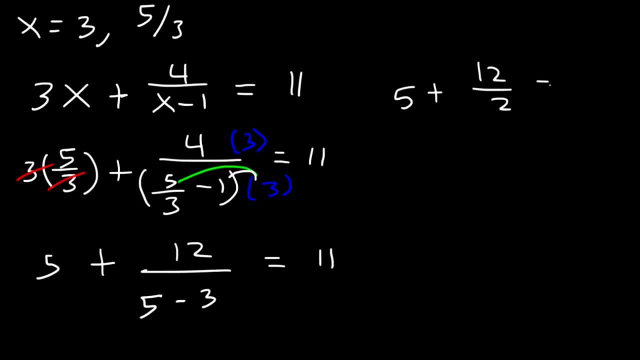 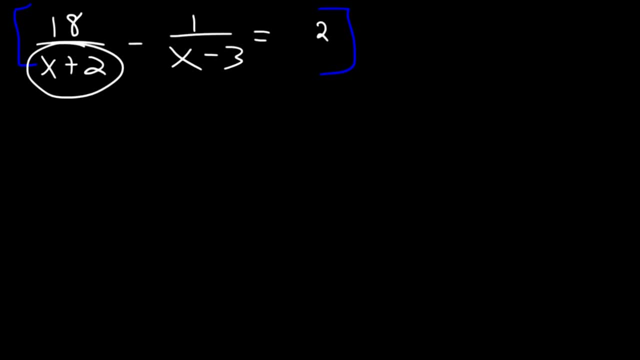 That is, by x plus 2 and by x minus 3.. So if we multiply the first fraction by x plus 2 times x minus 3, the x plus 2 term will cancel, leaving behind 18 times x minus 3.. 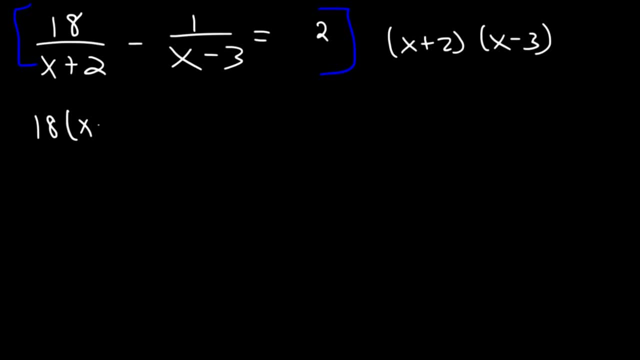 And that's what we're going to have initially. Next, if we take this fraction, multiply it by these two terms, the x minus 3 term will cancel, leaving behind 1 times x plus 2.. Or simply x plus 2.. 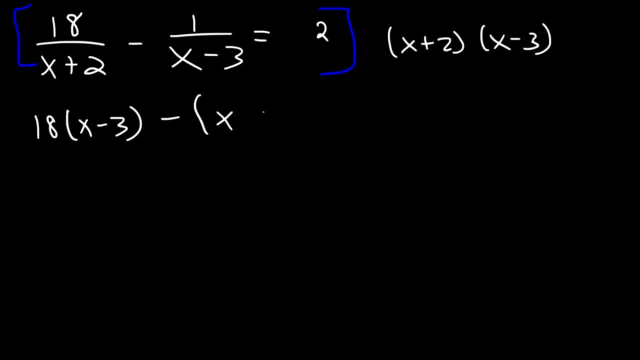 But don't forget to distribute the negative sign, which we'll do in the next step. And then, finally, we have 2 multiplied by these two terms, Or by those two factors, I should say. So that's going to be 2 times x plus 2 times x minus 3.. 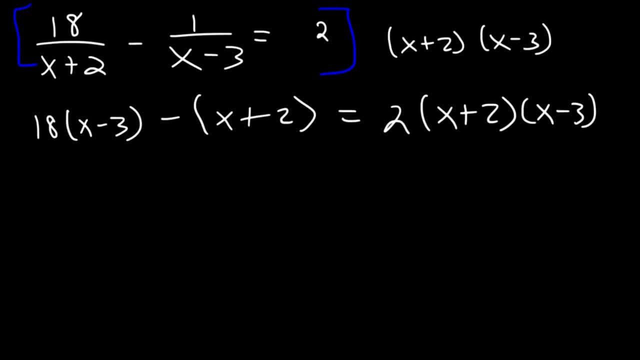 So now let's distribute FOIO and combine like terms: 18 times x, that's going to be 18x, And then 18x 18 times negative 3, that's negative 54. Distributing the negative sign, we're going to have negative x minus 2.. 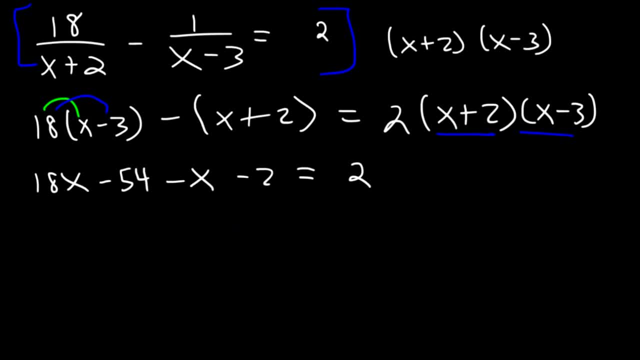 Next, let's FOIO these two factors. So first we have x times x, which is simply x squared, And then we have x times negative 3, so that's negative 3x, And then 2 times x, which is 2x. 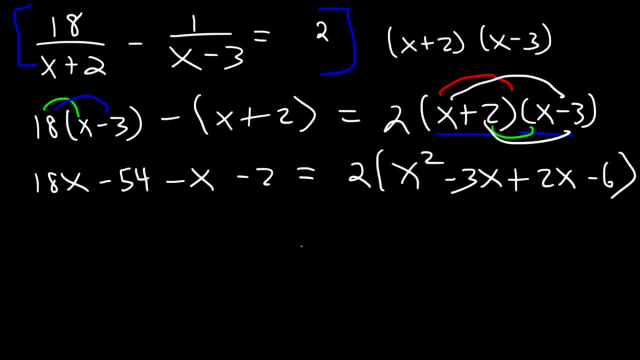 And finally, 2 times negative, 3,, which is minus 6.. Now, on the left side, we can combine these terms: 18 minus x is 17x, And we can also combine these two, which will give us negative 56.. 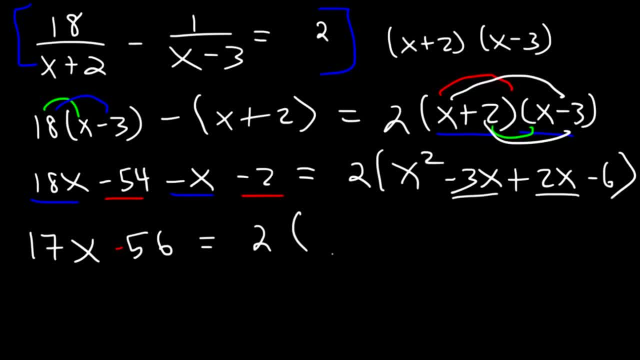 Here we can combine those two terms: Negative 3x plus 2x is negative 1x. Next let's distribute the 2.. So it's going to be 2x squared minus 2x minus 12.. So everything on the left side. let's move it to the right side. 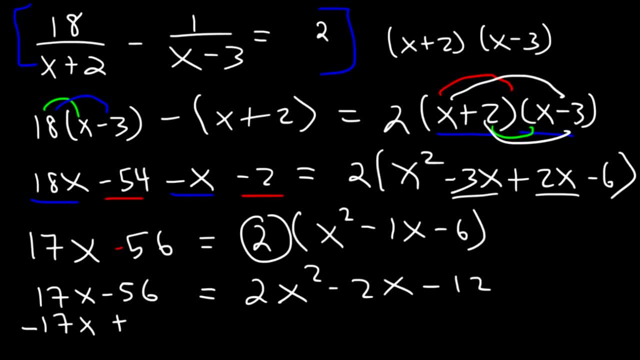 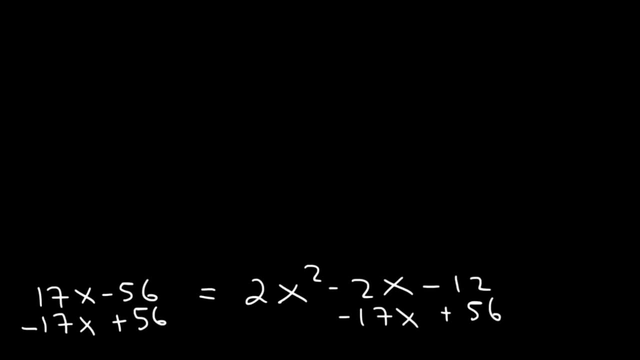 So let's subtract both sides by 17x And let's add 56 at the same time. So on the left we're going to have a 0. On the right it's going to be 2x squared minus 19x. 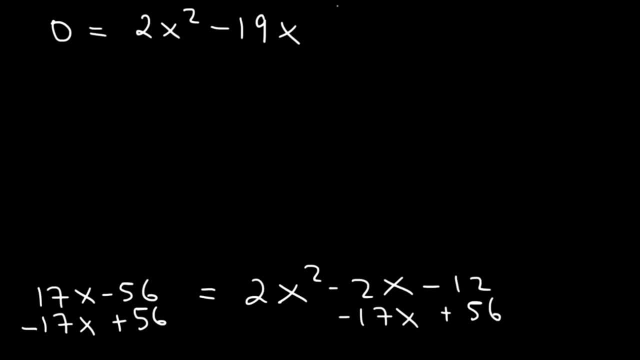 56 minus 12.. That is going to be 44.. Now we have another trinomial to factor And it's like the last one. So let's multiply 2 and 44. Which is going to? It's going to be 88.. 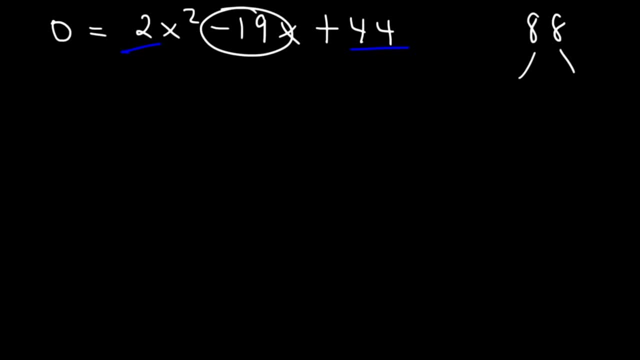 What two numbers that multiply to 88 but add to negative 19? Well, 88 is 8 times 11. And that adds to positive 19. So let's add two negative signs Now. let's replace negative 19x with negative 8x and negative 11x. 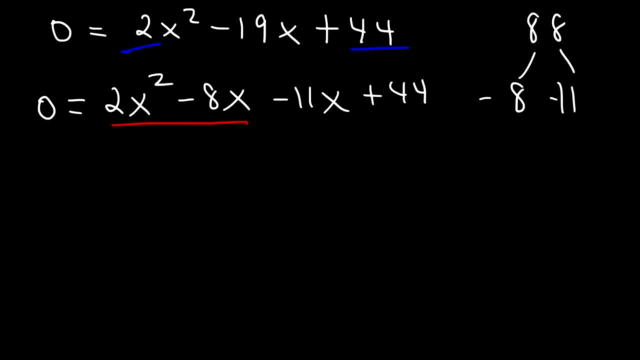 And then factor by grouping. In the first two terms, we can take out 2x, which will leave behind x minus 4.. And in the last two terms, we can take out 2x, which will leave behind x minus 4.. 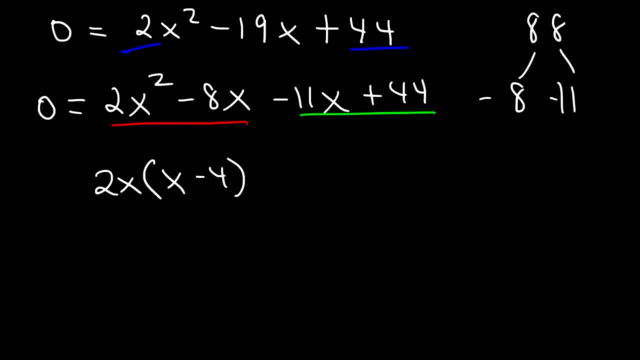 And in the last two terms the GCF is going to be negative 11x Or just negative 11.. And then we're going to have x minus 4.. So this is going to be x minus 4 times 2x minus 11.. 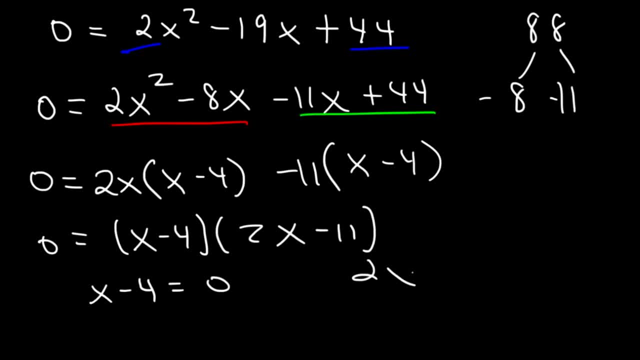 And now let's set each factor equal to 0. So we can see that x is going to equal 4.. And for the other one, if we add 11, then divide by 2, it's going to be 11 over 2.. 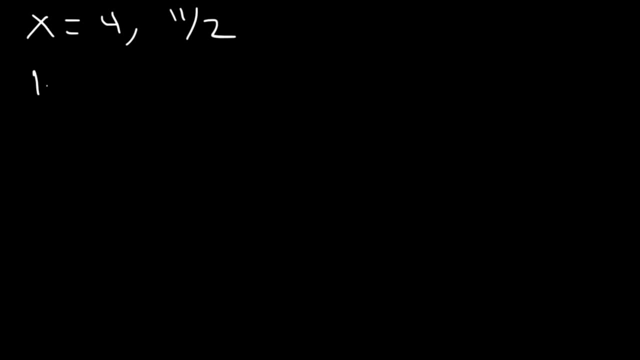 Now let's go back to the original equation And let's see if both of these answers indeed work. We have to make sure, though, because sometimes you may get an answer that doesn't work, And so you always should check for extraneous solutions. 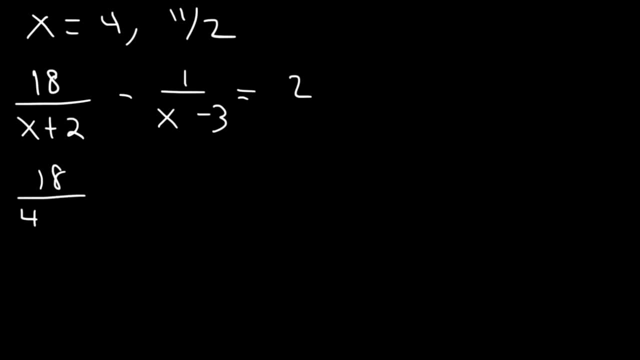 So let's start with 4.. So we're going to have 18 divided by 4 plus 2.. And then minus 1 over 4 minus 3.. Now 4 plus 2 is 6.. 4 minus 3 is 1.. 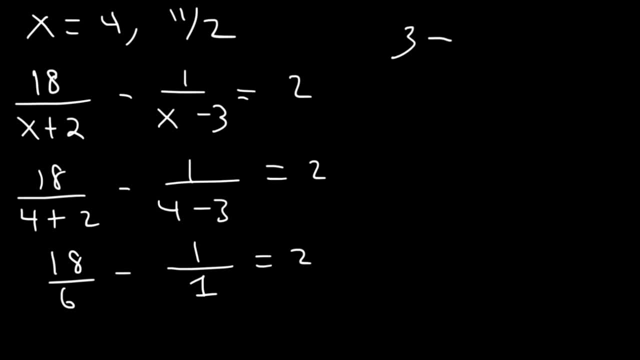 And 18 divided by 6 is 3.. 1 over 1 is just 1. And 3 minus 1 is 2.. So the first one works. Now let's go ahead and try the next one: 11 over 2.. 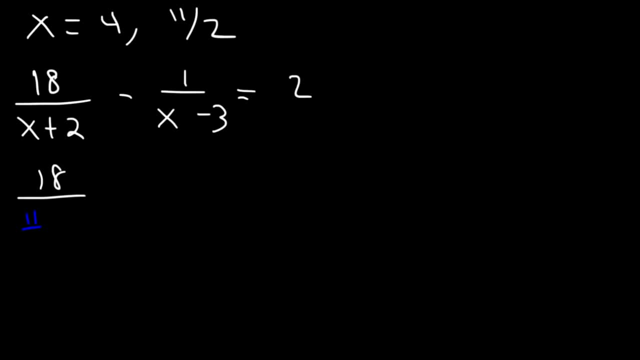 So it's going to be 18 divided by 2.. 11 over 2 plus 2.. And then minus 1 over 11 over 2 minus 3 equals 2.. So to simplify the complex fraction, let's multiply the top and the bottom by 2.. 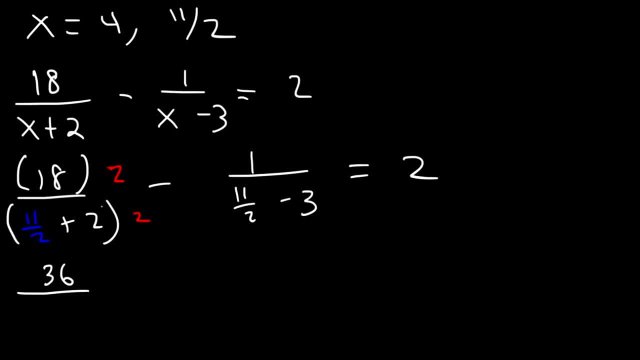 So 18 times 2 is 36.. 11 over 2 times 2.. The 2s will cancel giving you 11.. And 2 times 2 is 4.. For the other fraction, let's do the same thing. 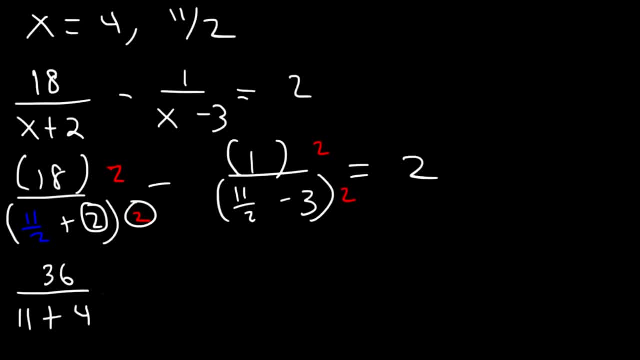 Let's multiply the top and the bottom by 2 over 2.. So on, top is going to be 2.. On the bottom we're going to have 11 minus 3 times 2 is 6.. All of this equals 2.. 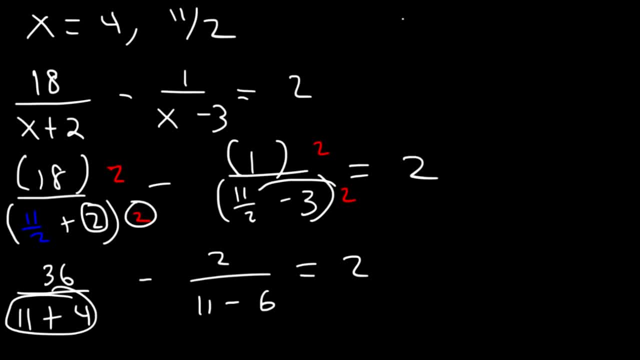 Now, 11 plus 4 is 15.. So we have 36 over 15.. 11 minus 6 is 5.. So this is 2 over 5.. Now to combine these, we need to get common denominators. Let's multiply the second fraction by 3 over 3.. 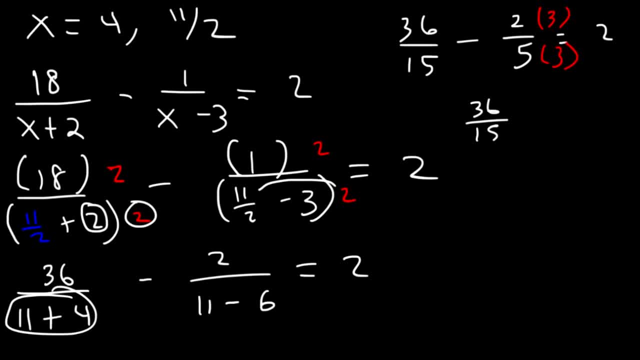 So this is going to be 36 over 15 minus 6 over 15.. 36 minus 6 is 30. And 30 divided by 15 is 2.. So both answers work in this equation. So now you know how to solve rational equations and you also know how to check them. 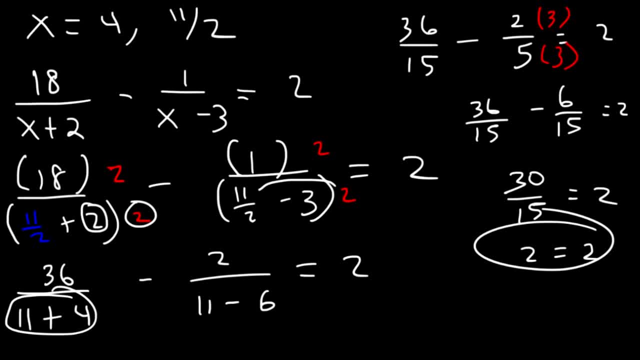 So that's it for this video. By the way, if you want to find more videos, check out my website, wwwvideo-tutornet, And you can find a playlist on algebra, trig, pre-cal, calculus, chemistry and physics. And you can also find that at my channel as well.